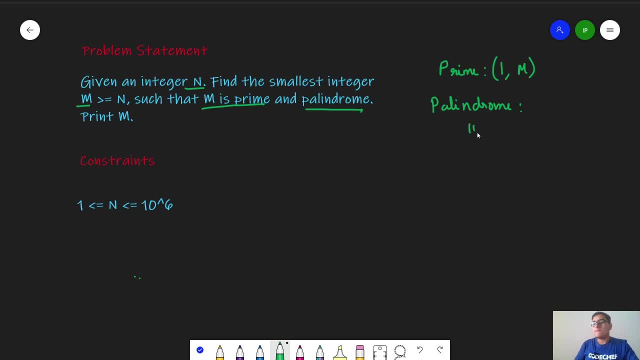 it reads same backward and forward, For example 101.. So if we read it forward or backward, it reads the same. Another example can be this or any other example. For primes, we have some common examples like 2,, 3,, 5,, 7 and so. 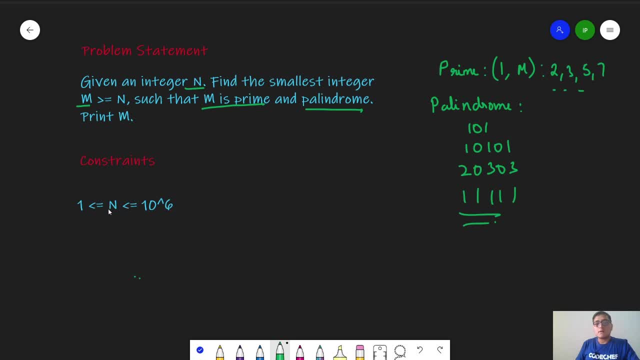 on. The constraints of the problem are: we are given n from 1 to 10 to the power 6.. Moving on to the test case, In the first test case we are given n as 31.. If we list out all the, 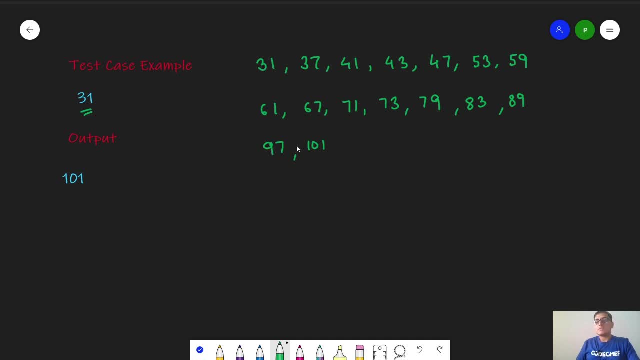 primes from 31 onwards, we will see that the first integer, which is a prime, is equal to a prime as well as a palindrome, is 101.. Hence in the output we have 101.. Moving on to the solution, The solution for this problem is pretty obvious. We will iterate from. i is: 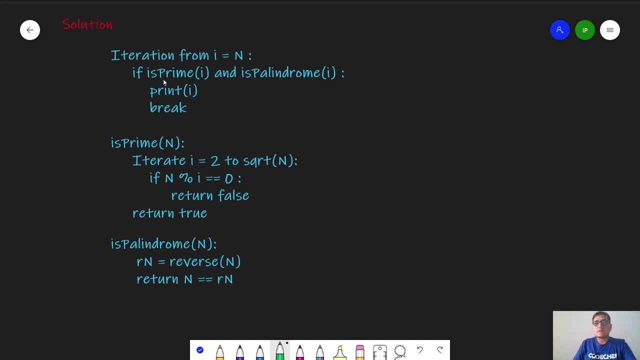 equal to n, to infinity. And if we find an i such that it is a prime as well as a palindrome, then we will pin that way i and we will break out, Else we will just keep on repeating this. Now, how to code the isPrime function. First of all, we need to know what is prime and 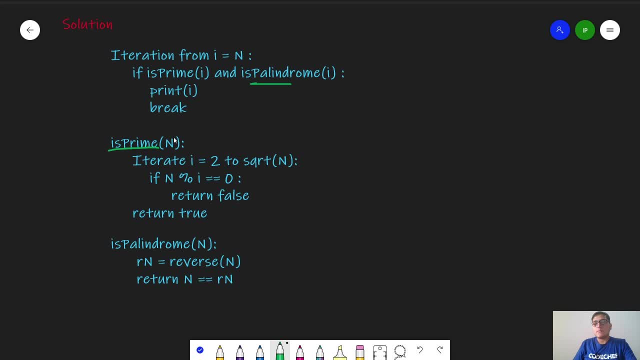 what is not prime. So we need to know what is prime and what is not prime. So we need to know what is prime and what is not prime. So we need to know what is prime and what is not prime To check whether a number is prime or not. we will iterate from 2 to square root. 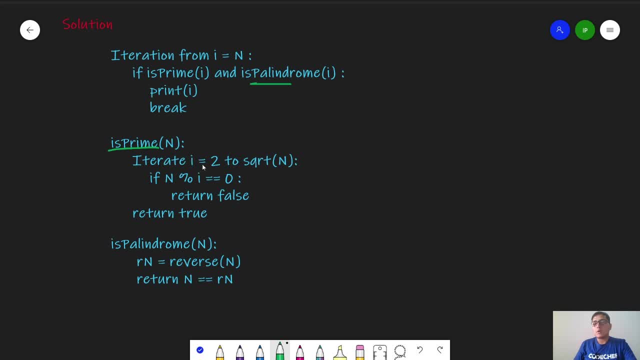 of n, and if any of the numbers from 2 to square root of n divides n, then we will return false. else we will return true. This is a pretty standard algorithm used to check prime numbers. The complexity of this function is square root of n, where n is given in the function. 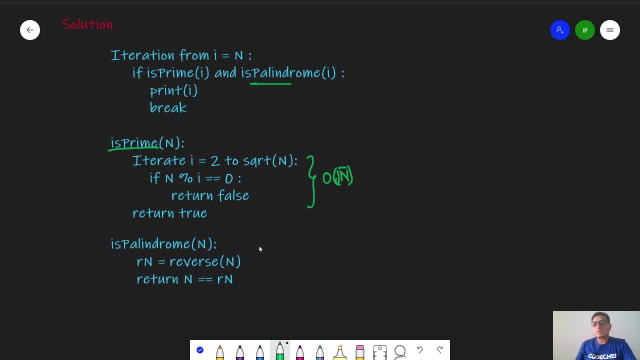 How to check a number is palindrome or not. For this we will convert n into a string and then we will find the reverse of this n into Rn and finally we will return whether the current string is equal to its reverse or not. The complexity of this is actually log of n. Why? Because we are given a bound. 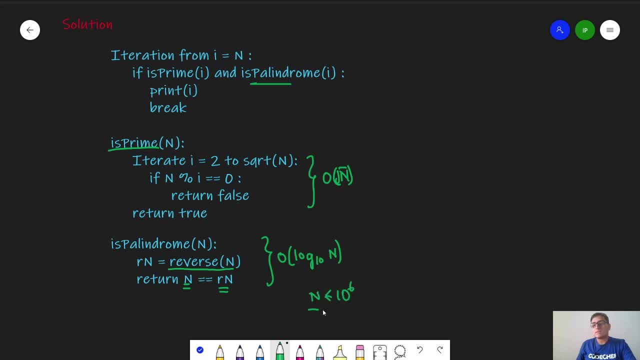 on n, that n is less than equal to 10 to the power 6.. So the length of n can be at most 7., Which is proportional to log of n. Moving on to the time complexity, Now it might look that you might run into infinity, but this is not the case, because for 10 to the power, 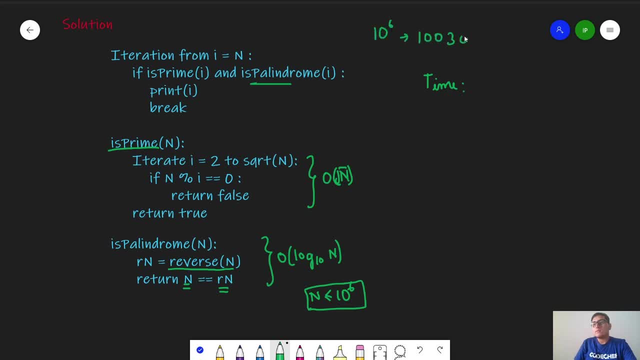 6, the answer is actually 1003001.. To find this, you can actually try a brute force solution and actually run for 10 to the power 6.. So the highest integer that you will ever check is 1003001.. 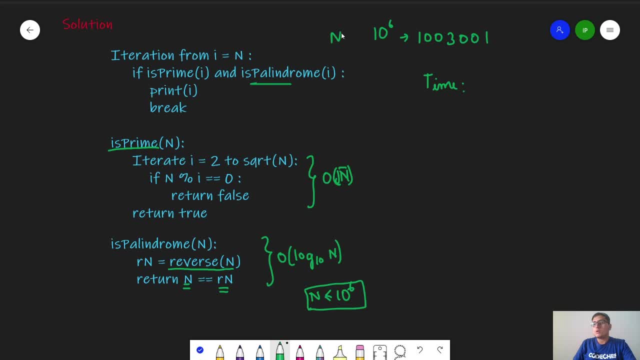 Which is proportional to 10, to the power 6 proportional to n. Hence our time. complexity is order of n root of n plus n log of n. This can actually be written as order of n root n. This is, however, a loose time, complexity a loose bound. The actual program will actually 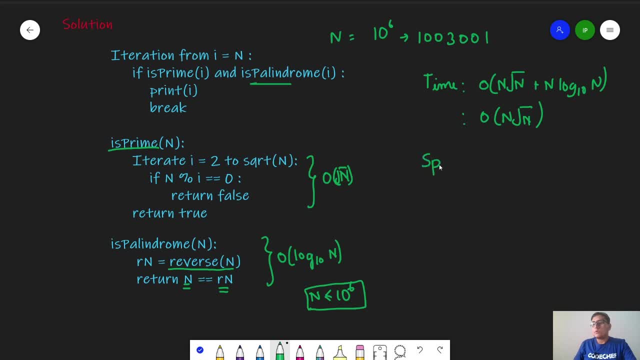 run very faster than this. The space complexity is order of 1.. Because we are only storing an integer n into an int variable and we do not store any other memory. So the space complexity is order of 1.. Moving on to the code, I have already taken the input into this variable n. Now I use 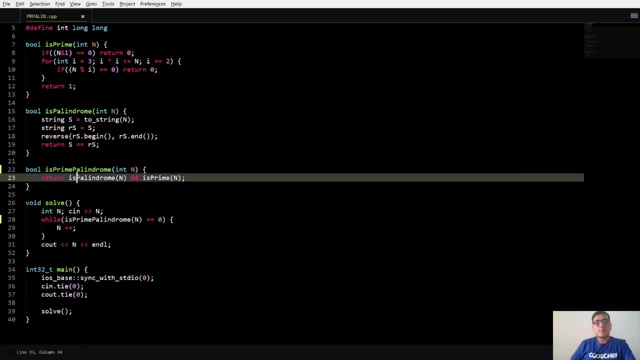 this function isPrimePalindrome to check whether the number is palindrome and prime or not. I use this inside of infinite while loop And I increment n accordingly if I want to. So I have already taken the input into this variable n. Now I use this function isPrimePalindrome. 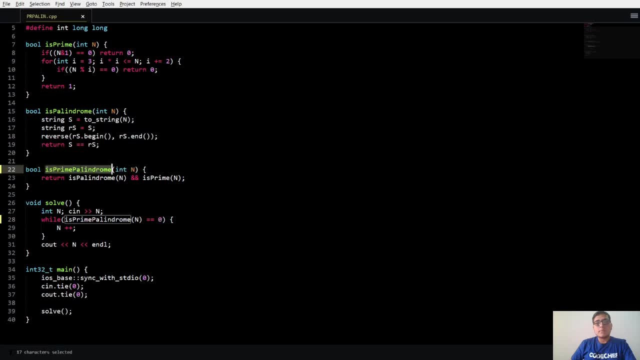 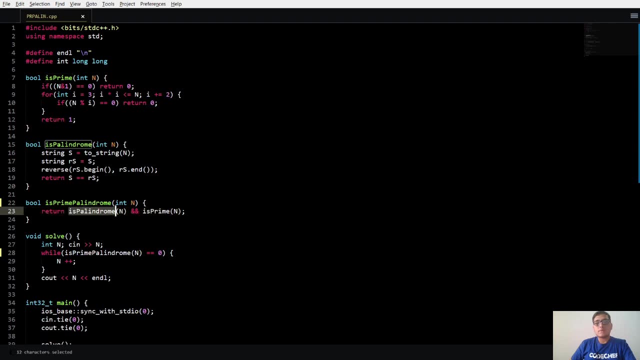 to check whether the number is palindrome and prime or not. I use this inside of infinite while loop. If the answer is no, isPrimePalindrome will check whether the number is palindrome and it is prime or not. It will return true only if both of the conditions are true. 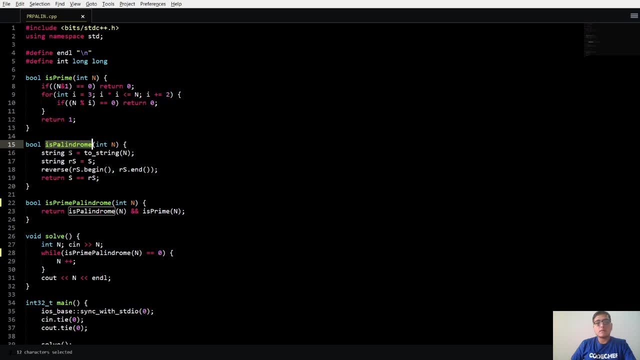 We will check palindrome using the technique discussed previously. We convert n into Smara and store the reverse of S into Rs and finally return whether S is equal to Rs or not, whether the string is equal to its reverse or not. To check a prime number, we will first check whether the number is even or not. If the number is even, then we just return 0.. Now we will iterate from 3 to root of n and check whether the number is divisible by any of the i or not. If it is, then we will return 0, which means that we will return false.